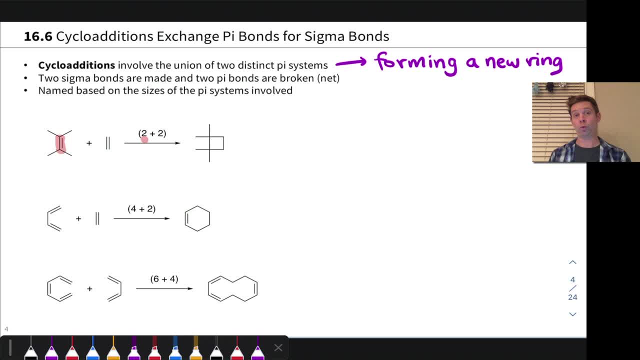 membered ring, and so here, for example, we have one of those highlighted in red, one highlighted in blue. we get those two coming together and the new sigma bonds are here and here. Electrons move, for example, from there to there and from this pi system back to the other. carbon. In the second case we have a 4 plus 2 cycloaddition, where this four atom pi system gets together and forms a new ring. This is how we name these pi systems. We end up with a six membered ring- again two new sigma bonds and notice that two pi bonds have been. 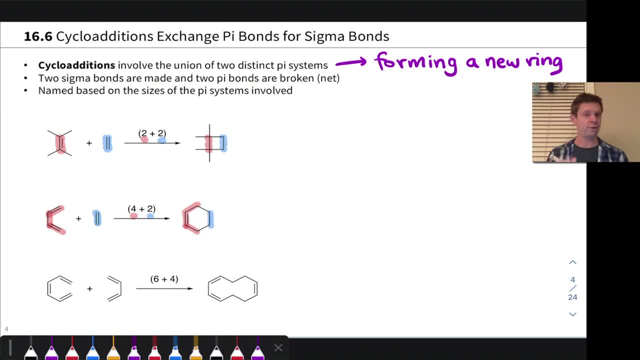 broken The pi bond in the blue two atom component and one of the pi bonds in the four atom component. Finally, we have an example of a six plus four cycloaddition, where a hexatriene gets together with butadiene and we end up with a ten membered ring. now where again? 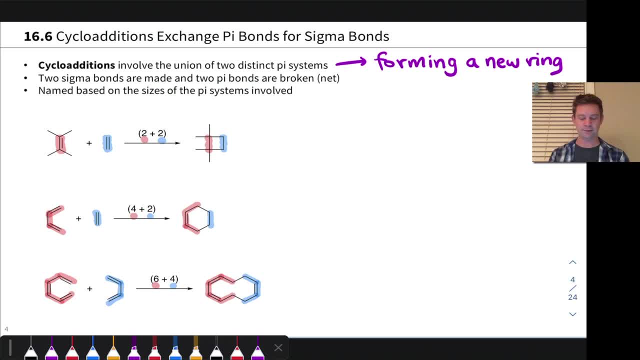 the two new bonds are between the termini or the ends of the pi system, and we've lost two pi systems, One from the six atom component and one from the four atom component. This four plus two, cycloaddition, is one of the most important reactions in all of organic chemistry and we're 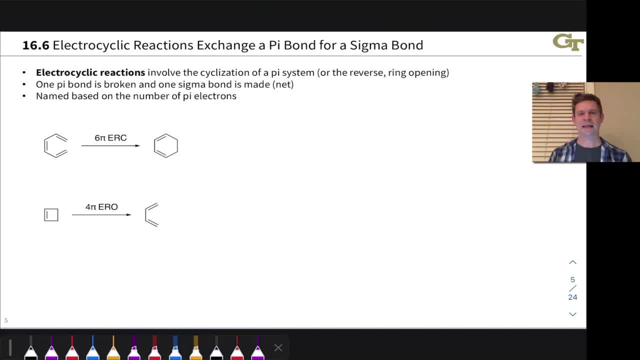 going to look at that in great detail in the ensuing videos. An electrocyclic reaction involves the cyclization of a pi system, or what we might call ring closing or the reverse, which is ring opening, to form a conjugated pi system. One pi bond is broken and one sigma bond is made. 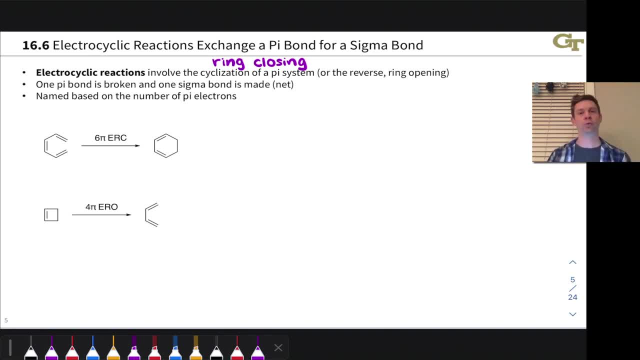 on the whole, although we're shifting pi electrons around, or pi electrons plus one sigma bond, to make these reactions happen, and these are named based on the number of pi electrons involved. So here at the top, for example, we have a six pi reaction where six pi electrons are moving around in a 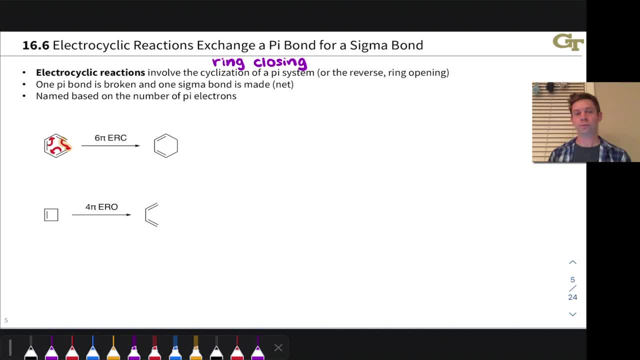 circle and the new sigma bond is really formed by this arrow highlighted in orange. So this is a six pi electrocyclic ring closing reaction At the bottom. here we have a four pi situation because there are four electrons shifting around and the one that breaks the sigma bond to open the ring. 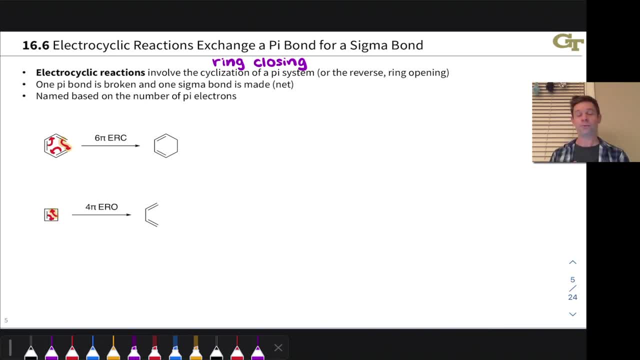 is really this arrow highlighted in orange right here. This is a four pi electrocyclic ring opening. Now, both of these are reversible processes. For example, this six membered ring could reopen back to the hexatriene system. This butadiene could hypothetically close to this four membered. 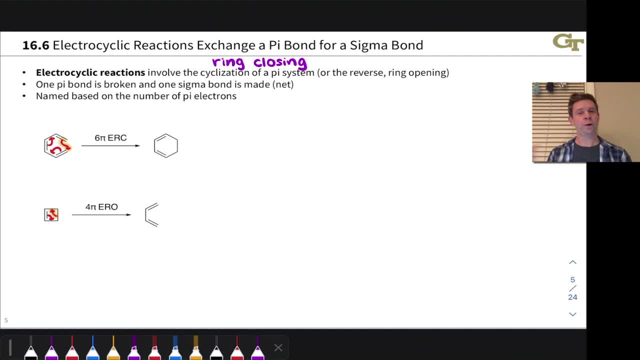 cyclobutene ring And in thinking about which side is favored, we want to consider things like ring strain, bonds made and broken and that sort of thing. So, for example, in this first case, this cyclization is often favorable because we're ending up with a six membered ring and we're 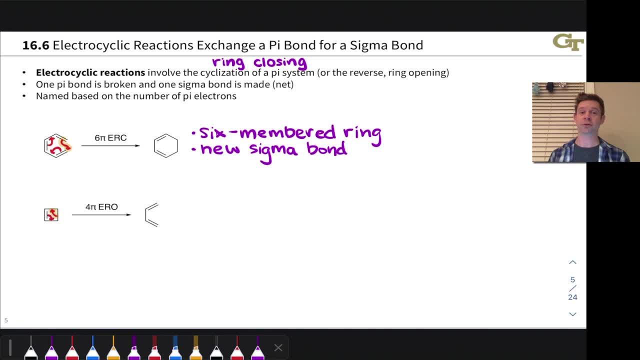 trading a new sigma bond for a pi bond, and sigma bonds generally being stronger than pi bonds, this tends to be a favorable process. In the bottom case, we are opening a four membered ring and so we're relieving quite a bit of ring strain in the cyclobutene, So this tends to favor the 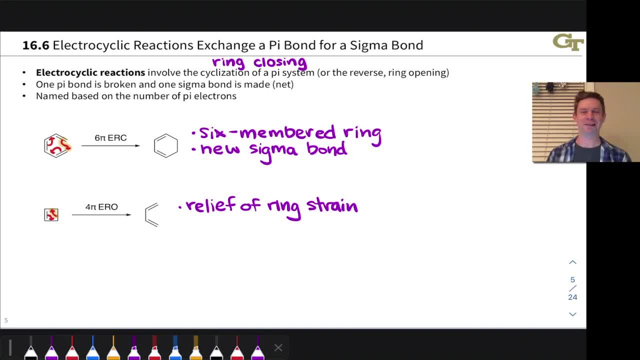 1,3-butadiene structure, which is not that favorable. So we're trading a new sigma bond for a pi bond. Not that surprising, given we've said a lot already about 1,3-butadiene. One last thing to consider here. 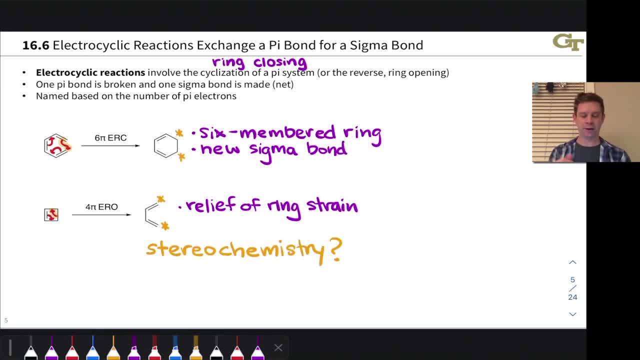 is stereochemistry. Electrocyclic reactions can form stereocenters, Both tetrahedral stereocenters when we're closing a ring and creating that new sigma bond, and trigonal stereocenters with EZ configurations, for example when we open a ring. So we'll talk a little bit more about. 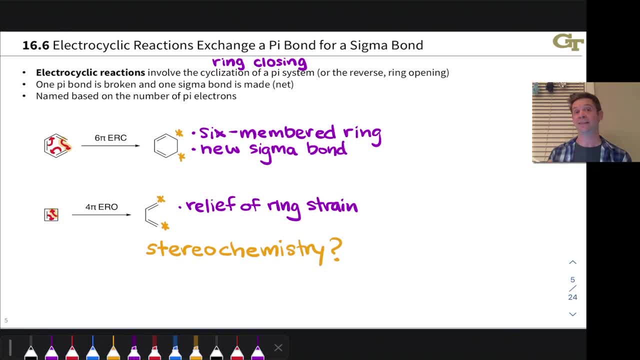 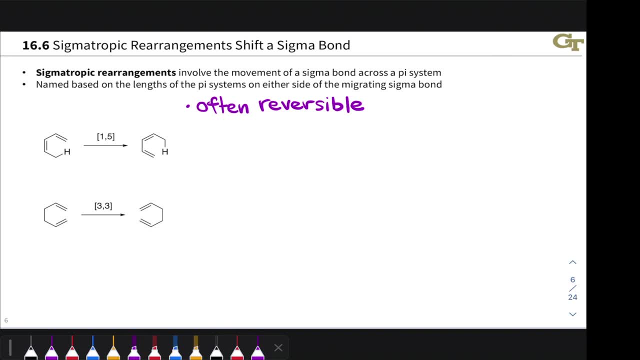 how to predict the stereochemistry of electrocyclic reactions in the near future. So, in a retropic rearrangement, a sigma bond moves across a pi system, and these are named based on the lengths of the pi system over which the sigma bond moves, And when a one is used there's no. 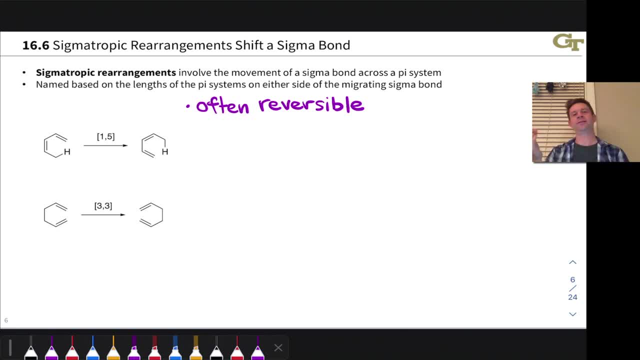 migration at all. There's just an atom that's moving with the sigma bonding electron sort of along for the ride as that bond migrates along a pi system of some length. These reactions are often reversible because there's no net cleavage or formation of sigma or pi bonds. So any 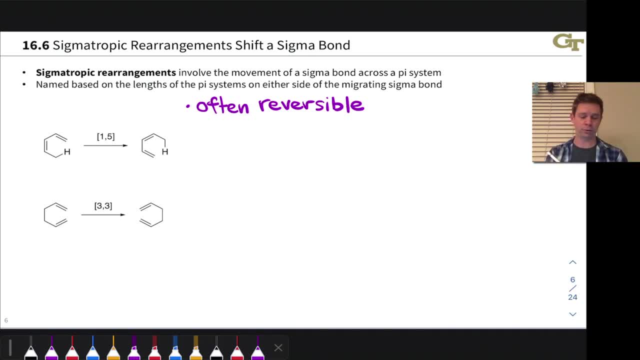 bias in one direction or another is going to come down to, for example, creating a more substituted double bond or a polarized double bond that's stronger than an unpolarized double bond that we start with in the starting materials, or something along those lines. The nomenclature: 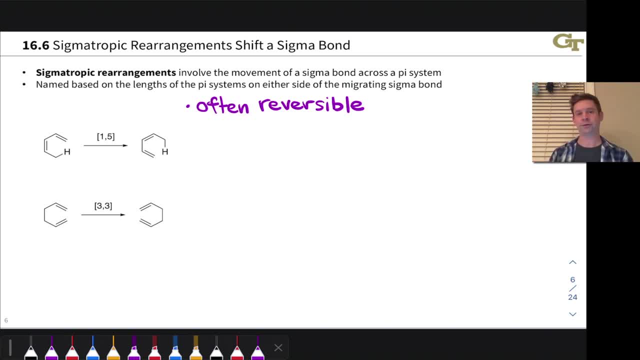 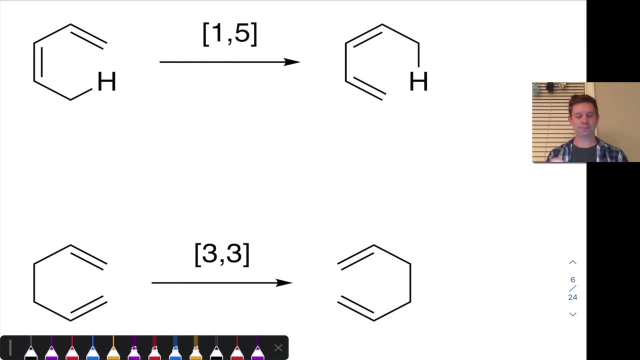 here can get a little bit confusing, and so I wanted to work through two examples of sigmatropic rearrangements to explain how the nomenclature comes about. First, here we have a 1,5 rearrangement at the top of the slide, and this is called. well, first let's look at the 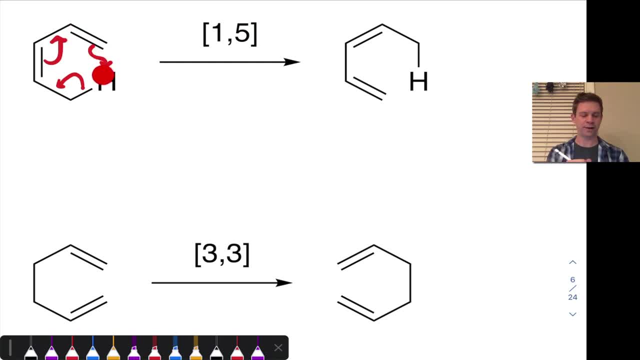 electron flow. So what's happening here is these pi electrons are heading into a new sigma bond with the hydrogen. you see that here, and then the C-H electrons are moving into a new pi bond and the pi electrons are shifting over to get us back where we started, in a sense. If we think about what this looks like, 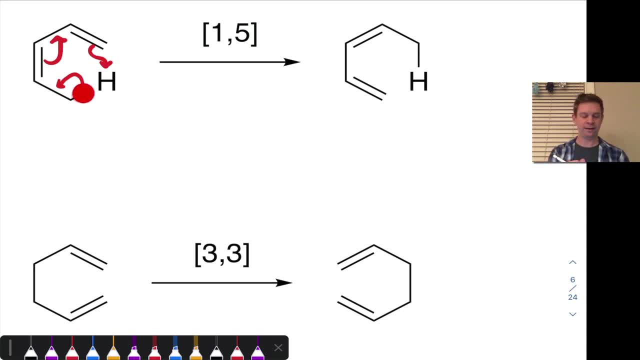 in terms of the migrating sigma bond. it looks like this sigma bond has moved from this position all the way to the other side of this pi system, which is 1, 2, 3, 4, 5 atoms. On the other hand, the hydrogen moved at all right, hydrogen has sort of just sat still. just come along for the ride with those. 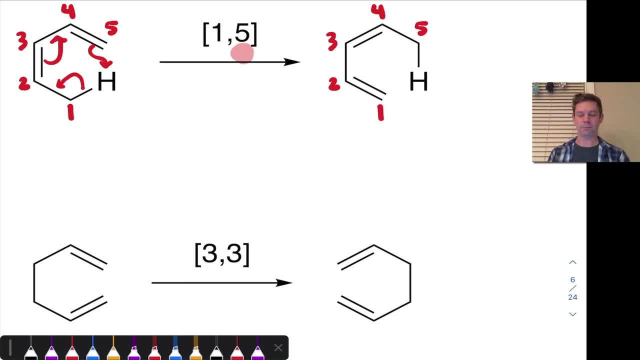 migrating electrons. and so there's our five atom pi system, quote unquote, from carbon one all the way around to carbon five. and that's where the five in this name comes from. but one comes from the fact that the other side of the bond doesn't really migrate anywhere, just sits attached to. 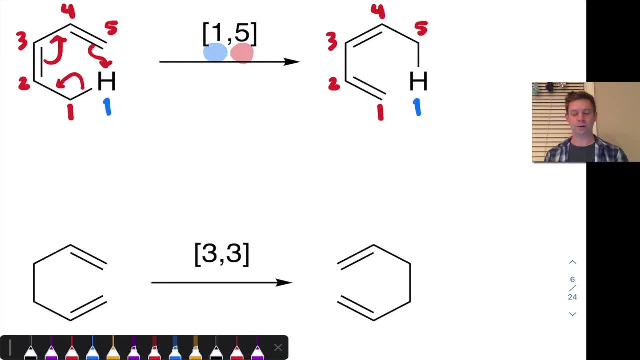 hydrogen the entire time. so this is a one five rearrangement. the bottom case is an example of a sigma bond migrating at both points or on both sides of the bond. what appears to happen here is this sigma bond moves over to this side both at both attachment points, right, and so this is what's. called a three. three sigmatropic rearrangement. the electron flow looks like this: it's again cyclic. so these pi electrons are used to create a new sigma bond. pi electrons shift over and the sigma bonding electrons break to form a new pi bond here and it's called a three. 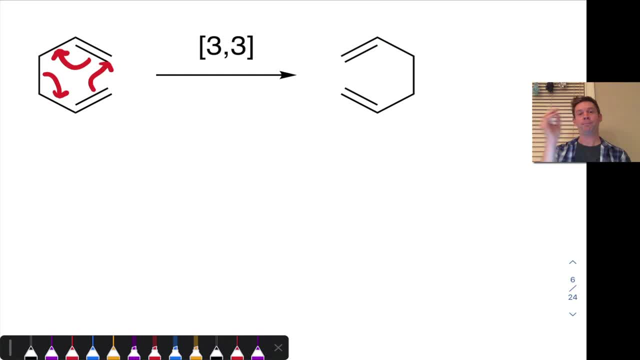 bond and the sigma bonding electrons break to form a new pi bond here and it's called a three- three because both ends of the sigma bond migrate over three atoms. so at the top, for example, we have one, two, three, and at the bottom we have one, two, three and notice that the new sigma bond 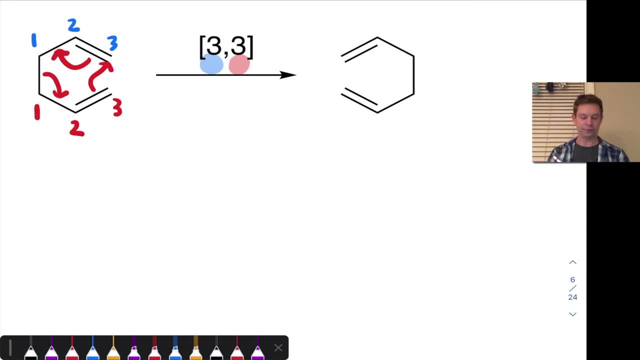 appears at carbons three and three on the other side. so let's go ahead and label those that side. we have carbon one, two, three and we have carbon one, two, three and this is called a three- three sigmatropic rearrangement because of the linkage between the two carbons labeled three in the product.